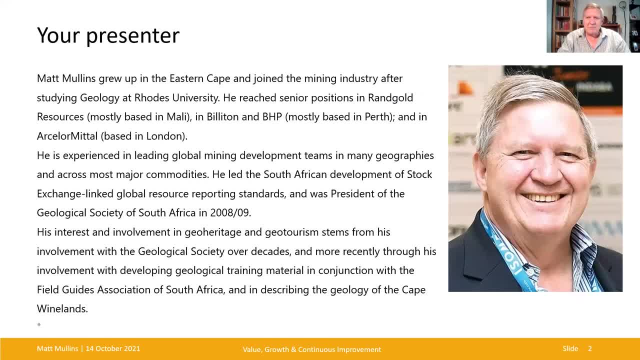 presentation To introduce myself. I grew up in the Eastern Cape and I do remember going for holidays down in Fisher River mouth and admiring the incredible rocks at the mouth there, which are the Dwaika Talat, wondering where the pebbles came from in the rock. And been told that I had a holy cross at the university最後 las tomas y el pedirim deseat grande edides, era de la posiblela que lo haya encontrado en los Lujos de la Escuela. Without being aeteen, what would you have하면, thought Wilson, How about knowing where thegotles came from in the rock and being told that there's an etwas eritreca del puerto que había una terania, que se ha puesto en la laceria, cerca del aper sampa? 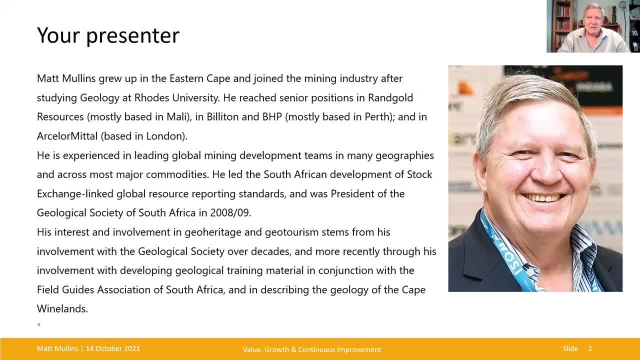 some of them would have been brought down by glaciers from many, many, many miles away, perhaps even as far as the Makroland, and wondering about them. I also remember playing in the more recent Aeolian Dunes, Solicified Dunes of the Bat's Caves, down at the Fish River Mouth. 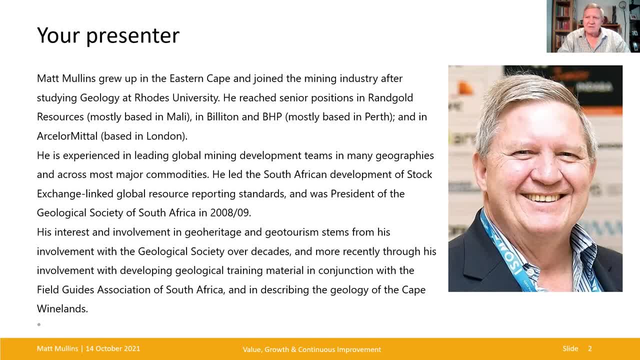 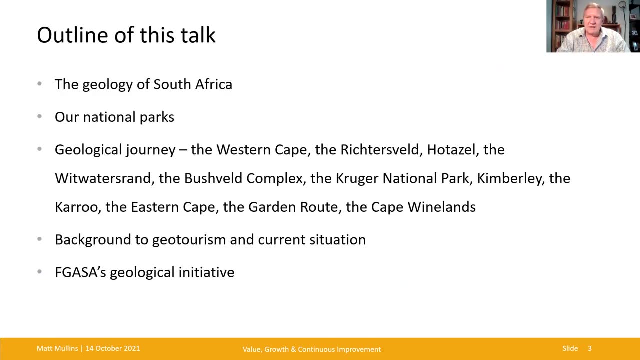 and wondering how the rock formed and that wonder has stayed with me to this day. I still look forward to my trips back to the Eastern Cape on a regular basis. The outline of this talk is: firstly, I'm going to talk about, very briefly, the geology of South Africa. 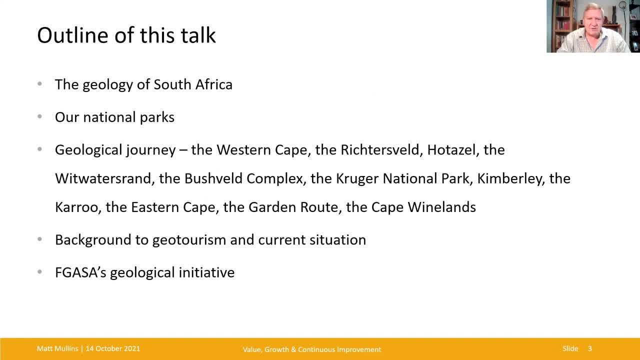 then touch on our national parks and how they fit in with the geology, then take you through a clockwise geological journey through South Africa. I'm going to start in the Western Cape, in Cape Town. move up north, touch on Hotazel. 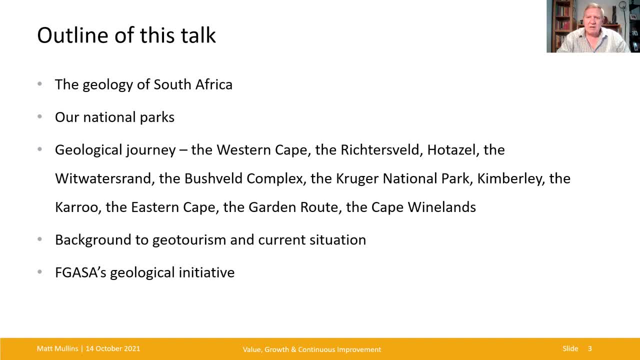 the Witwatersrand, the Bushveld Complex, have a quick look at the Kruger National Park, Kimberley itself, where diamonds were discovered. the Karoo. go down to the Eastern Cape, travel along the Garden Rope and back into the Cape Town area through the Cape Winelands. 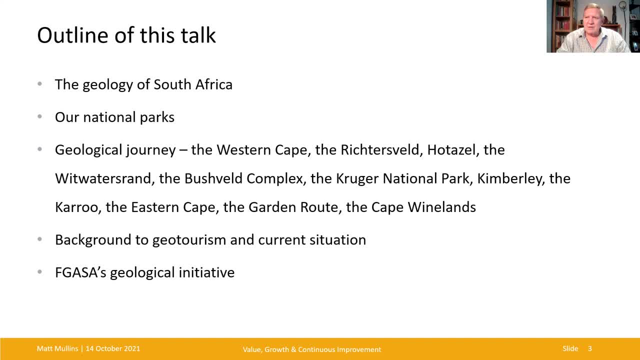 It is obviously a huge topic and I do apologise upfront for all of those fascinating and beautiful places that I will not be talking about but are just as interesting as the ones that I will be talking about. I'm going to finish off by looking at geotourism in general. 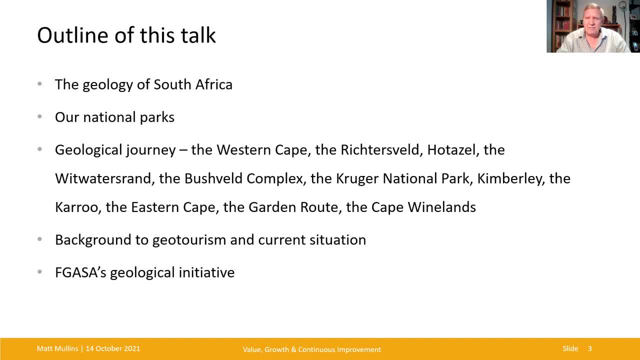 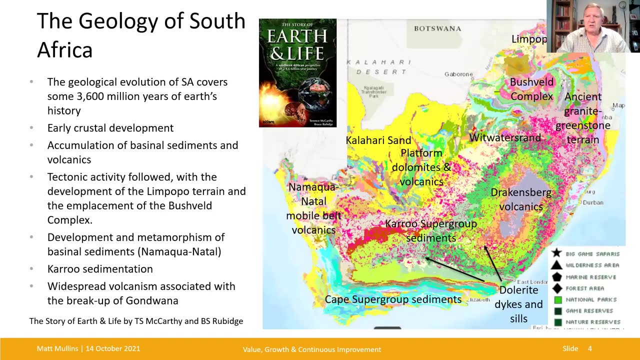 the current situation globally with respect to geotourism, and then finish off with talking about FGAS's very exciting geological initiative and our development of fieldguards and of a geological map. So let's turn straight to the geology- One of the nice things about geology. 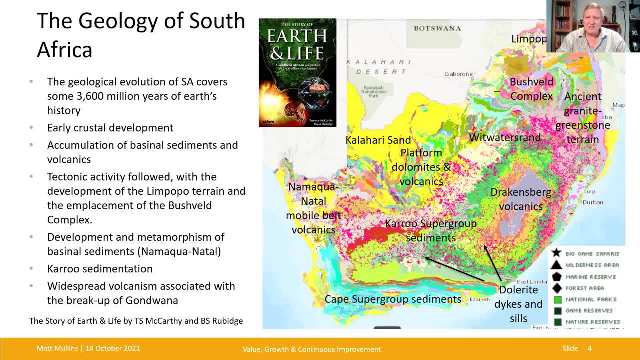 as is the same with many other professions is that you get to deal with very pretty maps. So the geological history of South Africa spans pretty much the whole of the history of the Earth. As you know, it's about four and a half to 4.6 billion years old. 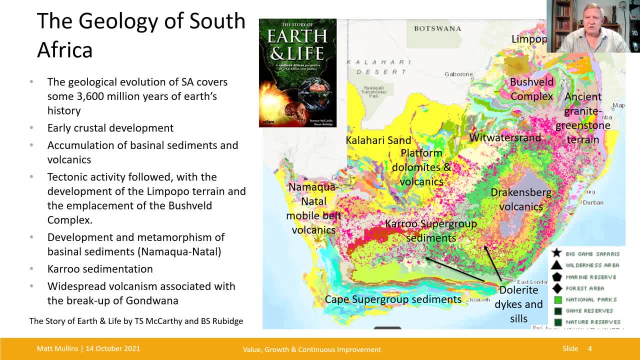 and we can identify rocks in South Africa dating back to about 3.6 billion years old. To simplify it, we can divide up the history of geological development mentioned in South Africa into six reasonably distinct but overlapping phases. Firstly, the development of early crusts. 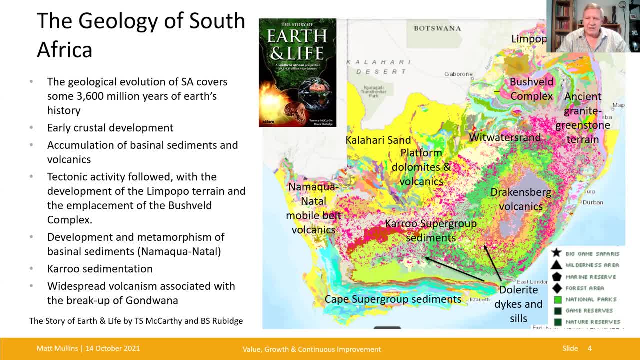 an early continental crust in the Barbiton area, where we know the wonderful granite greenstone terrains of the Barbiton Greenstone Belt, which is also where we have evidence of some of the earliest life discovered on Earth, dating back over three billion years. On that, we had crustaceans in the early 20th century, which is the site of the first geological discovery of the Earth, which is also where we have evidence of some of the earliest life discovered on Earth. which is also where we have evidence of some of the earliest life discovered on Earth. 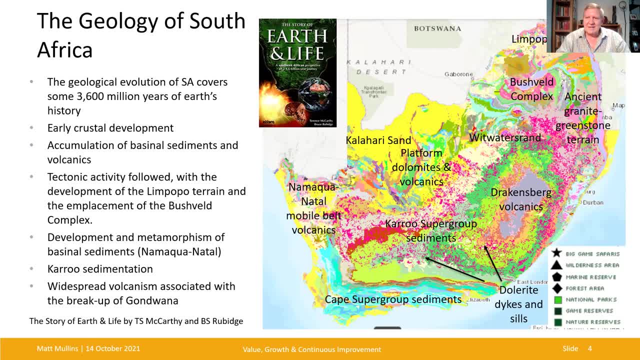 dating back over 3 billion years. on that we had crustaceans, crustal development extending the size of the early continental crust and the accumulation of basinal sediments and volcanics adjacent to those. tectonic activity followed after that with development of the popo terrain and the emplacement of the enormous bushville complex. still. 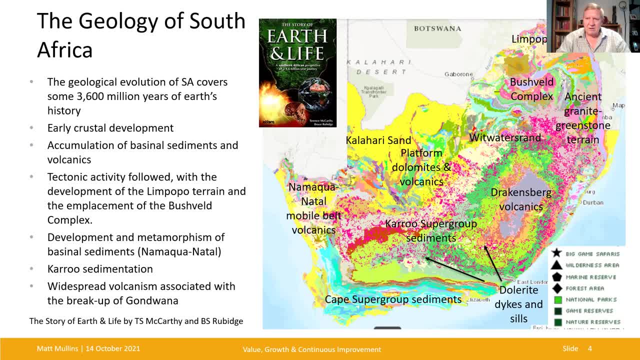 and is the biggest mafic complex ever discovered, with this powerhouse of minerals that it contains. after that, we had the development and the metamorphism of basinal sediments, we have the platform down dolomites and volcanics in the kuruman area and the development of 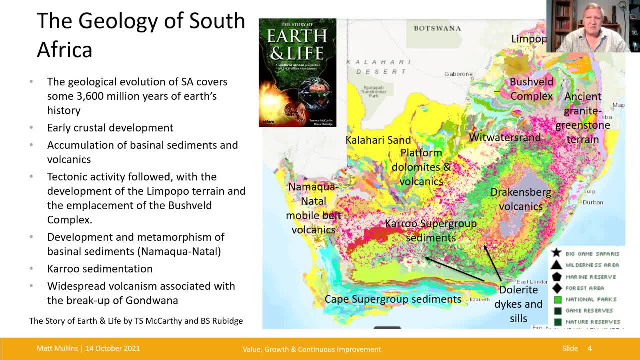 what we now call the namaqua natal mobile belt, sediments and volcanics and subsequent metamorphism. the largest event from a volume point of view was the karu sedimentation, which occurred around about when gondwana was in its heyday. we'll come to that. and that now covers 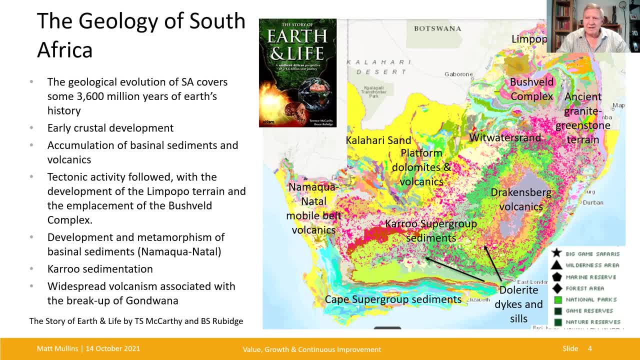 those sediments and associated rocks now cover two-thirds of the area of south africa. we then had widespread volcanism associated with the breakup of gondwana, forming the remnants of which we can see in the darkest burg today, but you can see in the little pink. 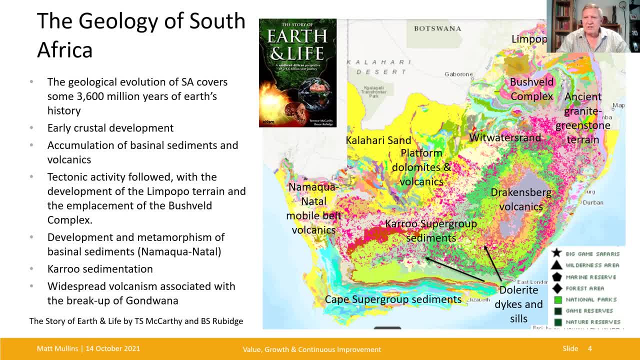 areas, the mass of dollarite ducks and sills which were the feeder ducks for the drops for volcanics, and you can see from the distribution of those that the volcanics would have covered much, if not most, of southern africa when that breakup occurred. and then, after the breakup, we've had the development. 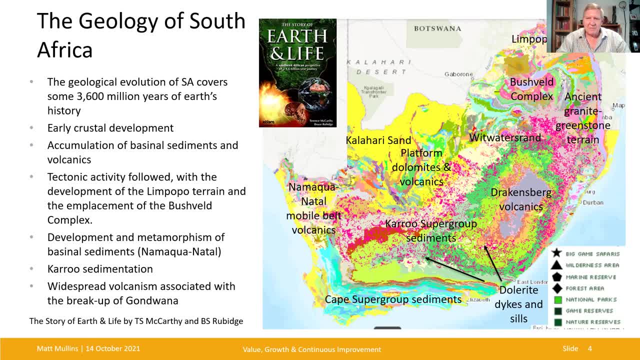 sediments and volcanics and coastal sediments adjacent to the current, the current areas. i'd like to you to have a look at a book that i've referred to there, called the story of earth and life and by spike mccarthy and bruce drewbridge, which is essential reading for 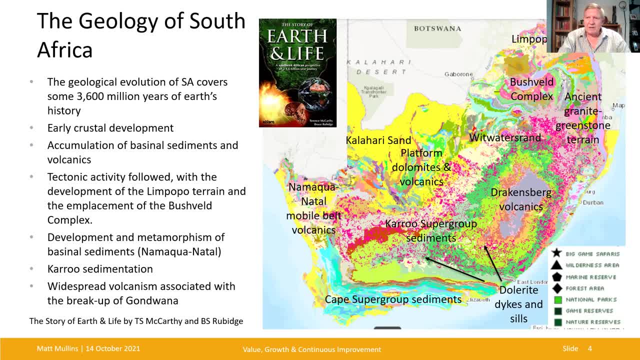 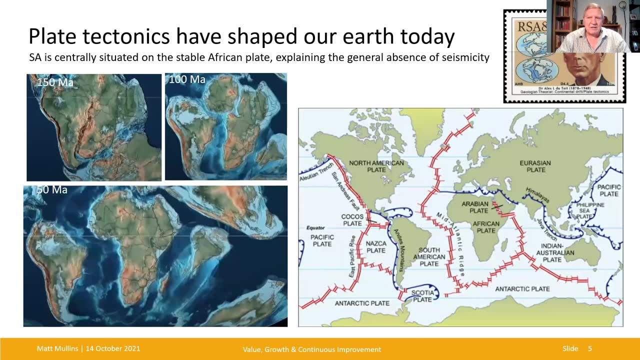 anyone who would like to look at how our earth, how our geology, developed in south africa and what we're looking at today. so no story of the development of south african geology is complete without looking at continental drift and what we now know as the theory of plate. 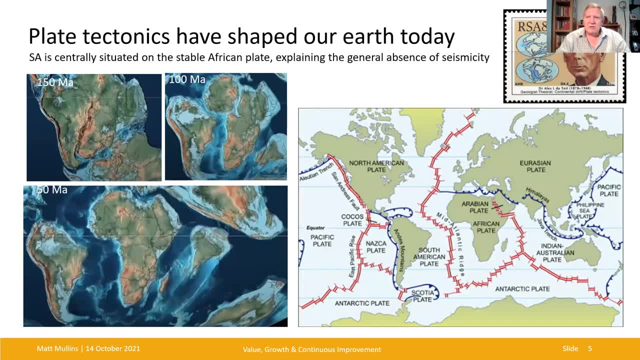 tectonics. the earth we know is composed of various crustal plates which are in constant motion with respect to each other. these have joined together and fragmented in past years. that it's really round about the sort of time that a super continent called pangaea came together around about 500 million years ago and 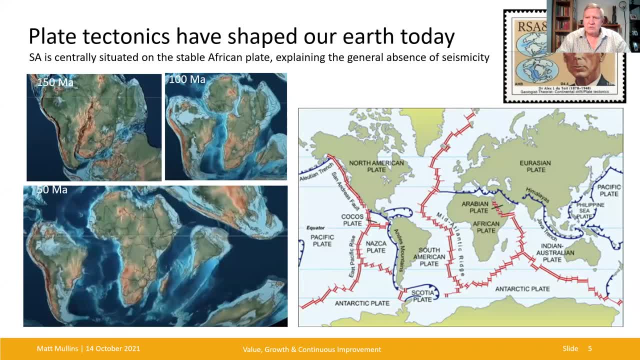 then started to break up, firstly into two siblings called laurasia and gondwana, and then gondwana started breaking up. so on the left hand side you can see the gondwana supercontinent, about 150 million years ago composed of south america, africa, australia, india and antarctica. with the breakup of 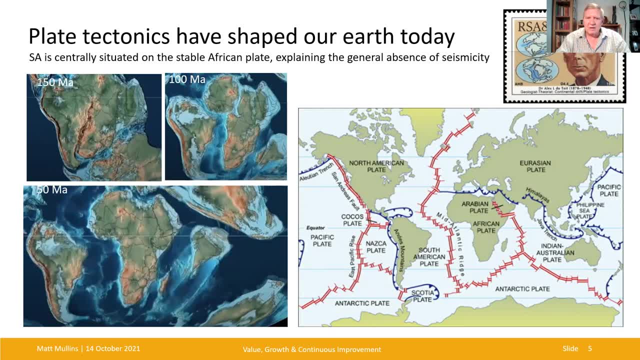 the gondwana supercontinent, south america started moving further to the west, the antarctica to the south, australia moved to its current position down under and india's started moving northwards, with madagascar just starting to break up from it. if you look at about. 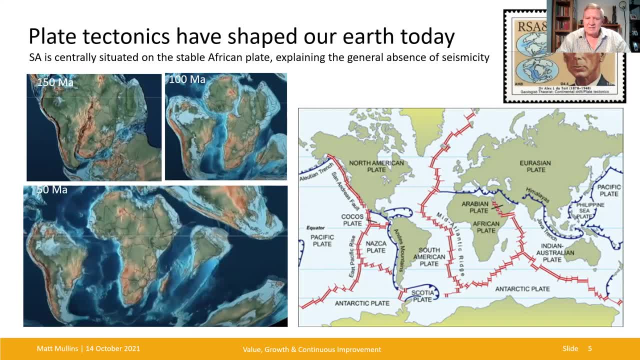 50 million years ago. you can see, the key things are: south america has started to move even further to the west and it's still moving westwards um. india, interestingly, has moved very quickly northwards and is in the process of barreling into asia, with that collision forming the himalayas as we know them today. 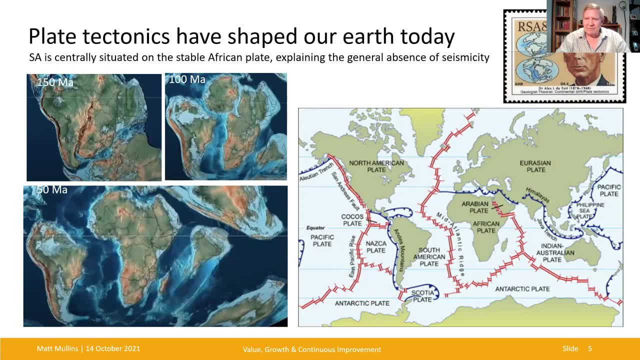 as we know them today, and antarctica and af and australia moving further apart. interestingly, the falkland islands used to be attached close to the african current coastline and that decided to move westwards and join up close to south america. we look at the current position with africa in the middle. it is on it. 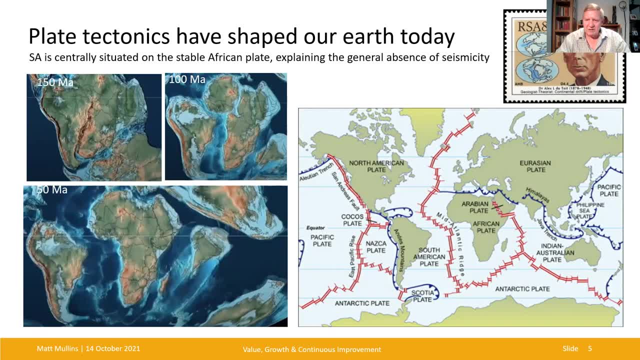 what we would call a tectonically very stable crash on, and that explains the general lack of seismicity and of the gondwana supercontinent- south america and the gondwana supercontinent- south america volcanism that we find not only in south africa but generally in africa compared to other areas. 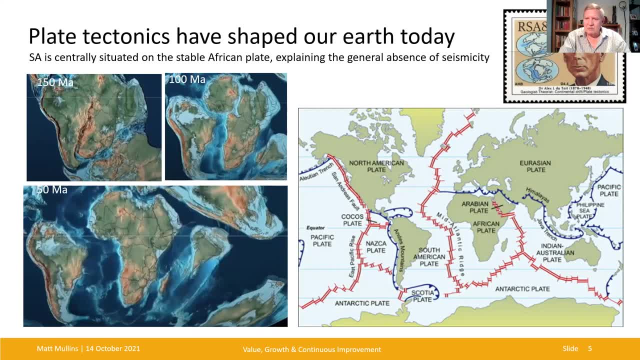 new crust has been created in the red areas- what we call the mid-ocean ridges- and has been consumed in the blue areas, and volcanism and seismicity tends to be associated with the red and blue areas, and recently we've seen some very spectacular volcanism in iceland. 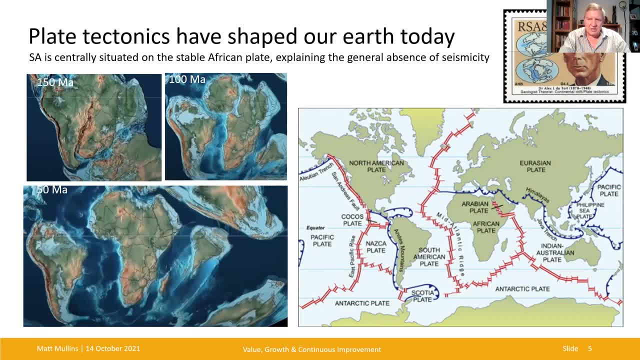 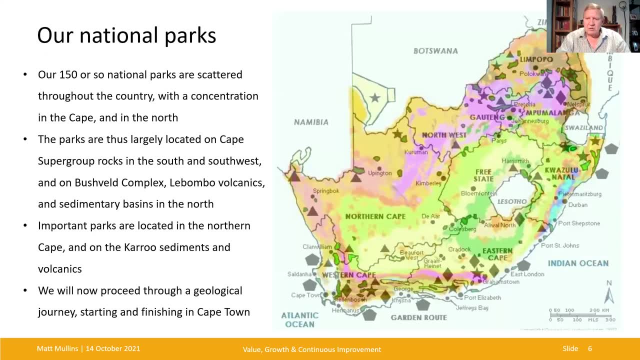 and down in the canary islands associated closely with the mid-ocean ridge. let's have a look at the next one. so i found our major national parks and various other parks. we see a preponderance and concentration of parks down in the cape, firstly in the western cape and secondly in the eastern cape and then secondly. we see a concentration. 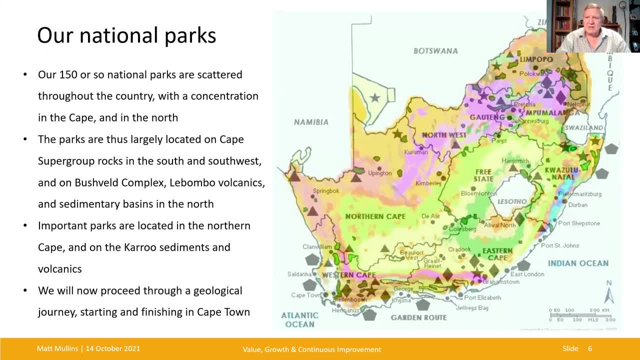 of parks up in the northern part of the country. the parks are driven largely by scenic beauty, by the geology that drives that scene, by the scenic beauty, by the occurrence of interesting flora and fauna and by the currents, as i said, of very interesting animals and the concentration of those animals in those particular. 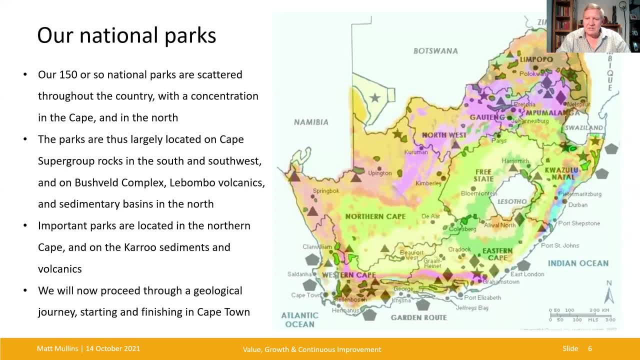 areas, and i include the bird life. that is not to say that other areas of south africa aren't just as interesting, but there are less numbers of parks in most of the karoo, for example, in the northern parts of the west of the country. we'll now look at a very quick geological journey through southern africa, and i'm not going to do it. 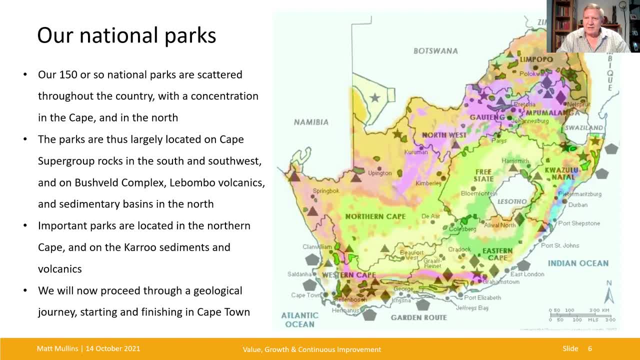 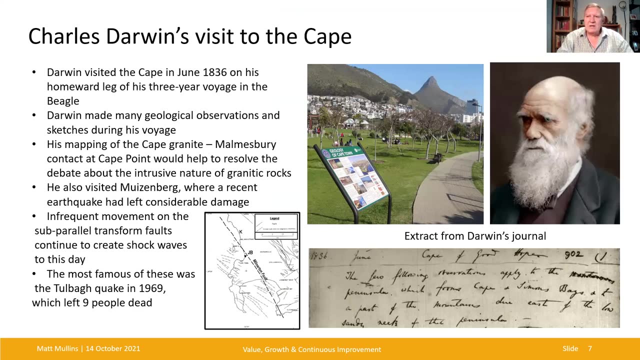 in geological time, but i'm certainly going to do it in geographical clockwise direction from the west all the way around the country. so let's start in cape town. that's where the mother city, where it all starts, and i'm going to talk about it as where geology starts. darwin is well known for his 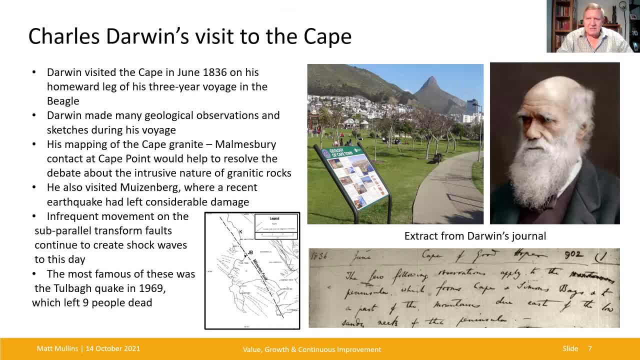 work on evolution and the origin of the species. what he is less well known for is his work on geology. he kept copious notes, as we know, and although apparently he didn't like studying geology, he ended up becoming a very, very good geologist. he visited the cape in june 1836. 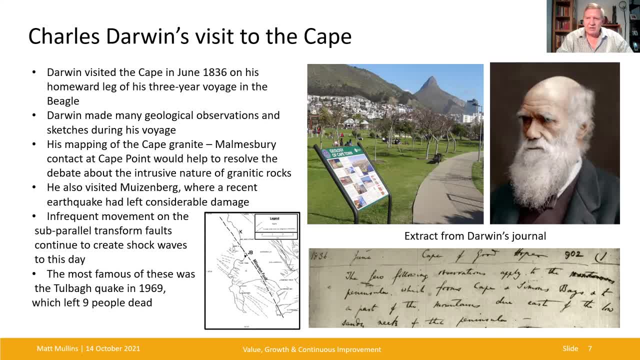 and made a number of observations on his visit there. one of them was the was to be a seminal observation on cape point, where his work on the intrusion of the granites into the malmsbury was helped to resolve a lot of the debate at the time on the nature of intrusive. 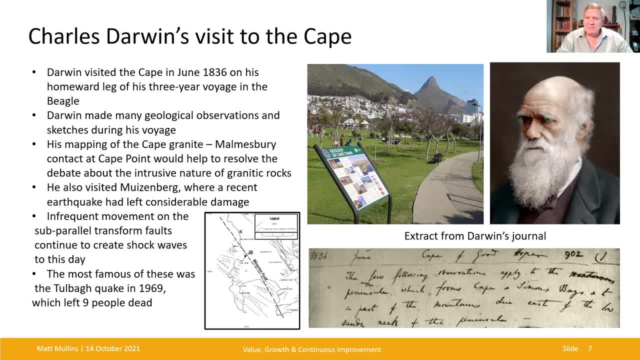 rocks. the other observations he made was visiting the damaged sand dunes in the middle of the area, or muesenberg area, where a recent earthquake had created a certain amount of damage. this is on the based on movement on the milderton fault, which even today we see movement in that area and occasional tremors. 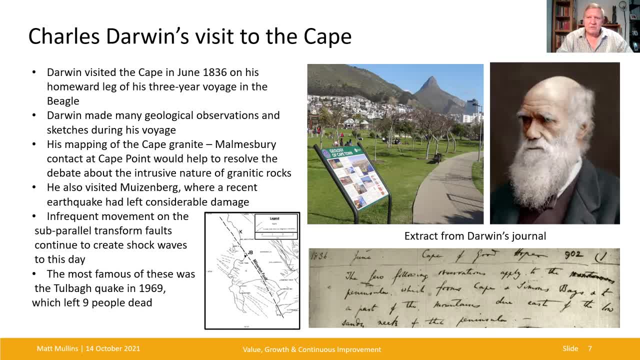 this is a sub-parallel fault- transform fault would call it- to the tulbagh fault, where we had biggest earthquake in south africa 1969, which left nine people dead. the bottom right hand corner you'll see an extract from darwin's diary and you'll see his his comments on his visit to the. 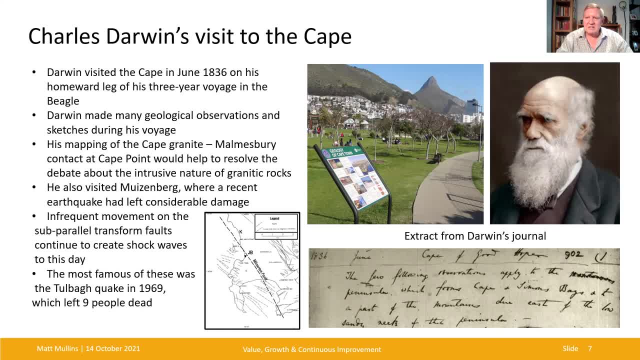 cape and in the middle of you'll see a very excellent geo plug that's been erected on green point and i encourage all of you who can go and visit it to go and have a look at that and have a look at the description of the geology of cape town in that plot. we move from there to 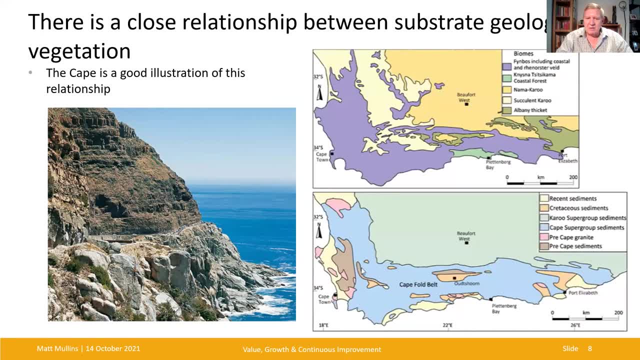 down towards cape point, the chapman's peak drive which we know well, showing the granites on the bottom side and the sediments of the cape super group sitting above that. what i want to highlight in this particular start is the very close relationship between vegetation, or biomes, and 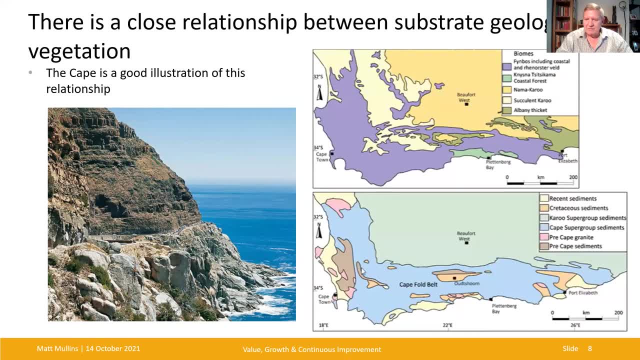 the geology and you can see the cape fall belt itself shown in light blue at the bottom. the cape super group sediments been very closely associated with the fame fanbos biomes and as we move north into the karu, shown in the green as the karu super group sediments, we move very 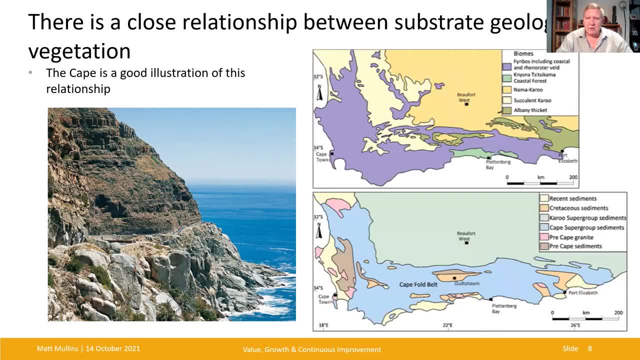 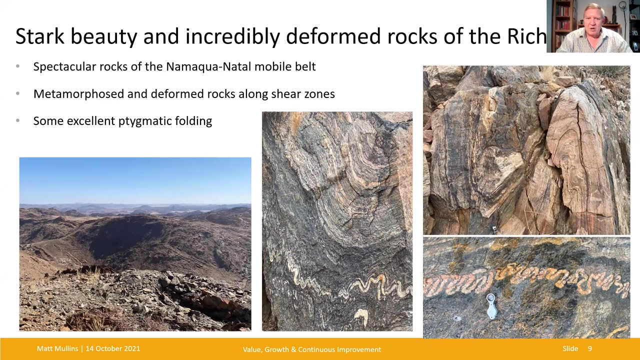 quickly into different biomes, the normal karu biome. this relationship we can see throughout the country, and although climate plays a large part in what biome develops, the substrate geology also has a big part to play in dictating what the vegetation is like. let's go even further north, up into the heart of the namaqua natal mobile belt. 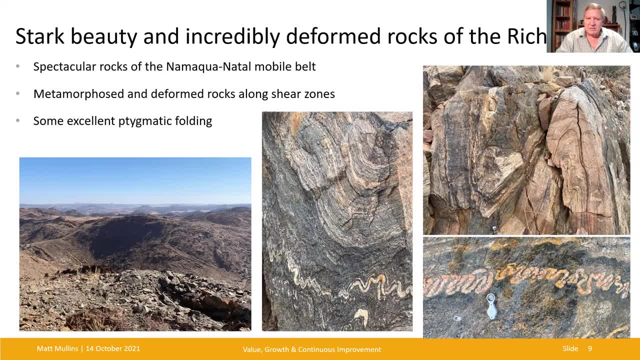 and you've seen on the left a picture there of, uh, just near the orange river, i think five kilometers from the orange river. we're looking northwards there and you get these linear east-west trending shear zones, of which the poor father shear zone is probably the most spectacular. we have lateral movement on the rocks. as the rocks moved, they 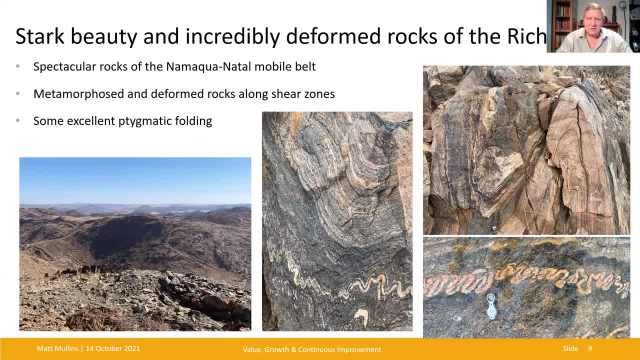 were became plastic. they were probably still fairly hot and they created these spectacular folds, as you can see. on the right, the very tight ice carnal, almost folding, and some very, very interesting tegmatic folding where the density contrast has created a very interesting scribbly rock. i'll call it almost looks like ancient writing. 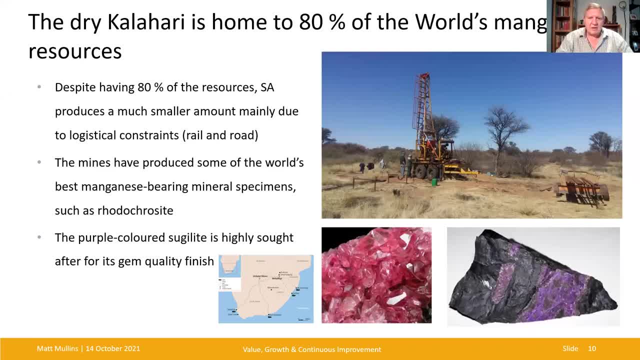 we move to hotazel, where approximately 80 percent of the world's manganese resources are contained in the hot cell manganese field. you can see a drilling rig on the right-hand side and you can see a stone in their height on second engagement plate. sure, what you think is some. 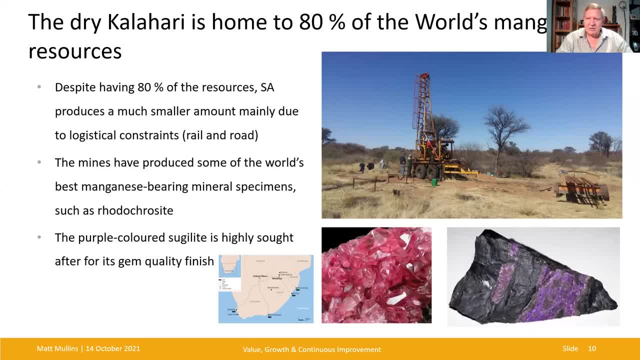 really interestinginki. Luego of the settlement in bandswitch, much of what you and who do is working very carefully to mitigate the there in the, the pinkish color that's rhodochrosite, which is one of the really really special manganese minerals, and also the one on the right hand side which is called sujalite. 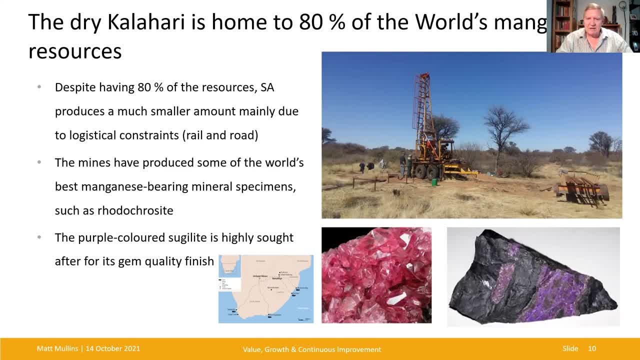 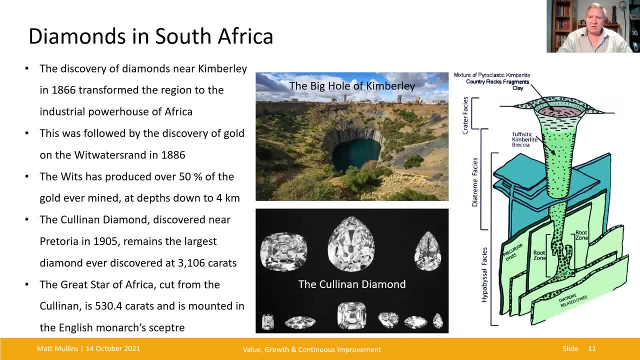 or vesalite, originally from the vessels mine where it was discovered and it's a highly, highly sought after mineral force gem quality finish. moving to further to the east, we have where diamonds were discovered. the discovery of diamonds at close to kimberly in 1866 transformed south africa from a fairly 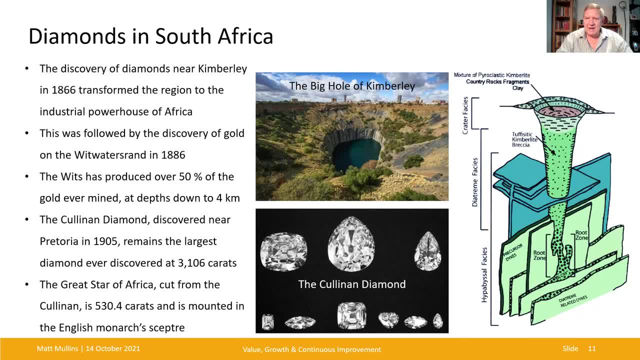 agriculturally based backwater with a staging post down in cape town for passing ships, to what it is today, a, an intellectual powerhouse and the biggest economy in africa. we'll see the big hole there. the cullinan diamond was actually found near pretoria and that's still the biggest diamond. 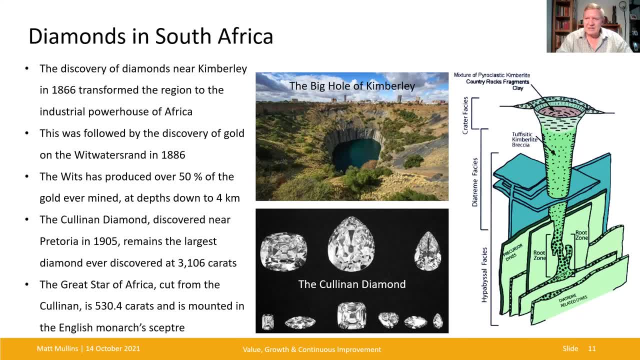 that's been found in the world at three thousand one hundred and six carats, and the one diamond, which is the staff, the greatest of africa, was cut from the cullinan. it's 530 carats and it's mounted in the english monarch scepter. on the right-hand side you can see a schematic of how a diamond pipe forms. 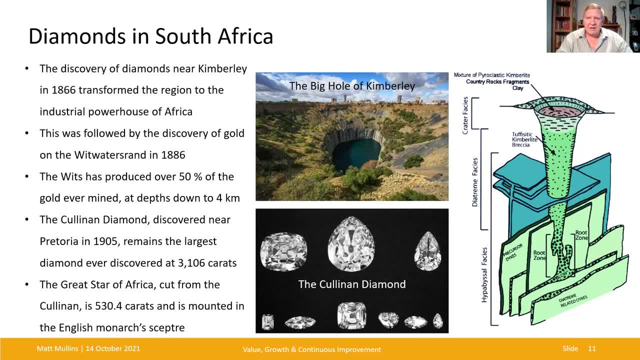 and you can imagine, with the surface only covering a couple of hectares, how difficult it is to form. it's also very soft on surface. it tends to be covered by other sedimentary after eruption and that is why it also becomes very, very hard to form. We should also remember 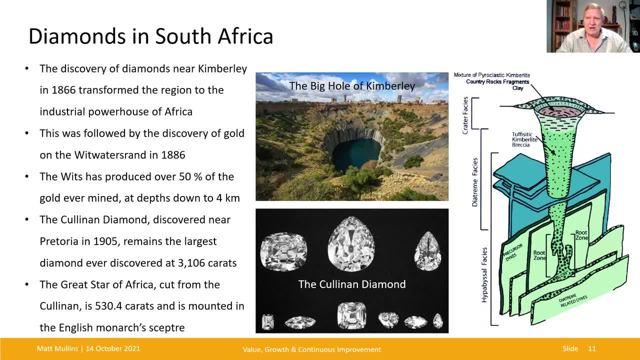 that diamonds have played a major part in some of the exploration of Africa and in South Africa we have many instances of shipwrecks along especially the wild coast and the southern cape coast, where carrying diamonds from India to Portugal and many legends of diamond farms and many legends of diamonds that are still to be found along that coastline from those shipwrecks. 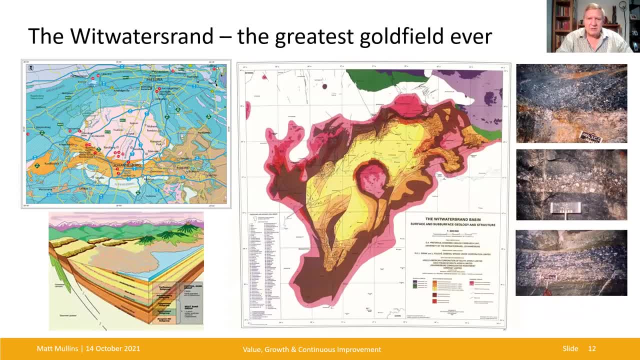 We move to the fabulous Witwatersrand. Most of the wits is covered by surface rocks. so you'll see, on the left, top left, you'll have the pinkish color- is the granite dome which covers much of Johannesburg, and draped along the southern part of the dome are the Witwatersrand rocks. 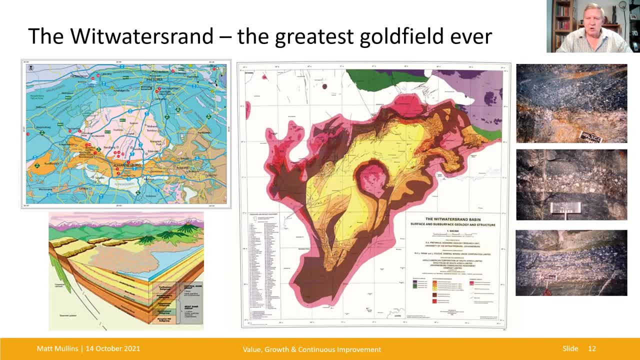 and very, a very small part of the rocks are actually exposed around there and in other parts of South Africa. In the center part of that slide you'll see what looks like the Witwatersrand basin looks like with all of the cover rocks removed and you can see that. 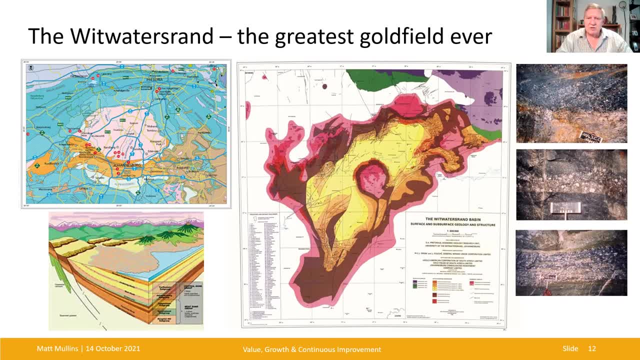 it's actually a huge wits basin stretching 350 kilometers by about 200 kilometers, and that pinkish zone in the middle is the Friede Fork dome, which is interpreted as being the result of a massive, massive meteorite impact approximately 2 billion years ago. You can also see the 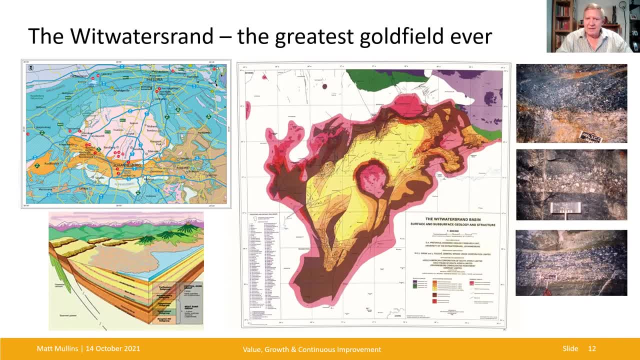 Johannesburg dome arrowed there, and on the left hand side, in the bottom, you can see the development of the sedimentary basin and the interpretation of how the difference with Witwatersrand reefs actually falls. The right hand side are some illustrations of the conglomerate reefs and, just as a reminder, 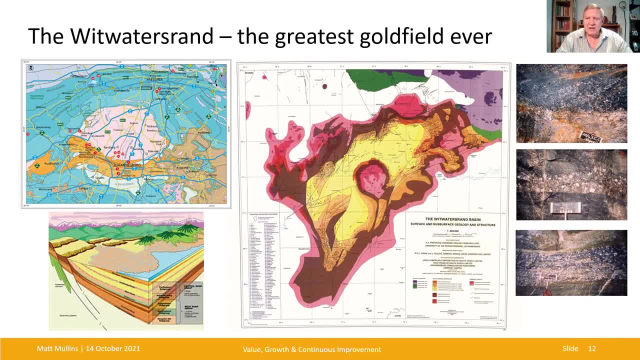 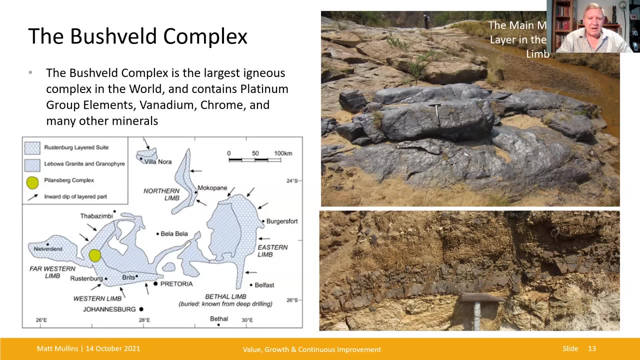 over 50 percent of the gold ever mined in the world has come out of this particular sedimentary basin- Still a phenomenal basin, and it's like it's never been found elsewhere in the world. Let's move into the Bushveldt, also a minerals powerhouse, and when it's the largest. 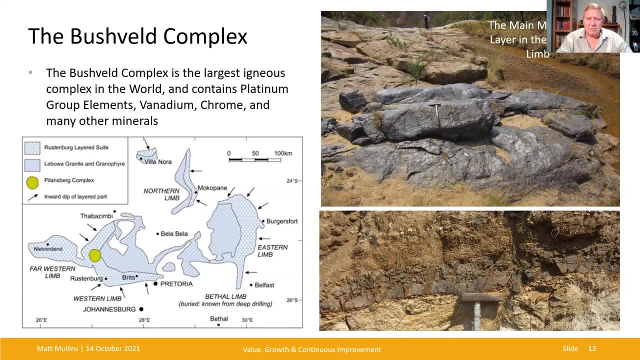 mafic complex in the world. you can see its outcrop shown in the bottom left hand all the way from Litvedind, Tabazimbi, Mokopani Burgers, Fort Belfast and down to Pretoria. It actually is enormous, contains pretty much- I think 60 to 70 percent of the world's platinum. 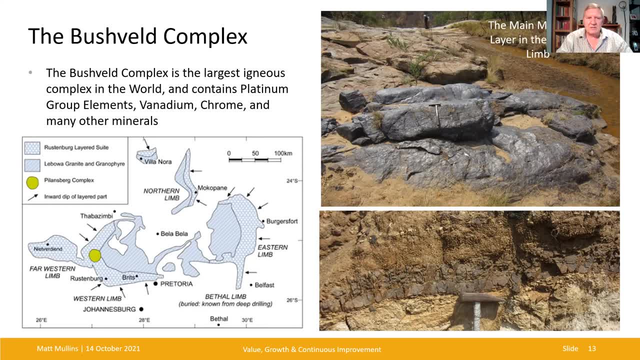 group minerals, but also contains enormous amounts of vanadium, chrome and many other minerals. One of the most important things is that it's not well known that near Tabazimbi we have the world's biggest deposit of andalusite, which is used in refractory minerals. On the right hand side you'll. 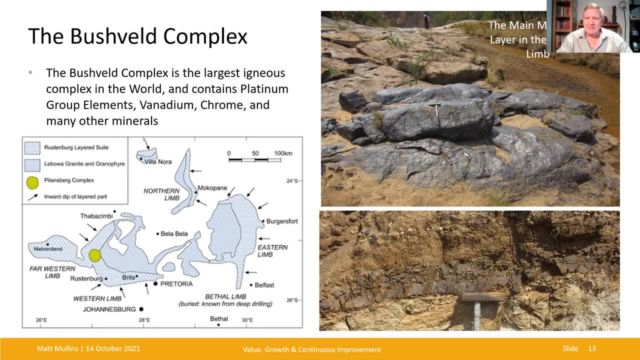 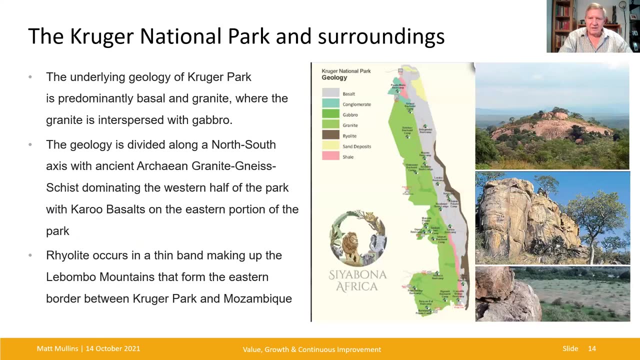 see the main magnetite layer, which is chocoblock, full of, firstly, iron, as you would expect, but of vanadium, and that shows, on the bottom right hand side, the thickness of the main magnetite layer of about a meter or so. As I said, full of vanadium in it. Let's move over to the Kruger Park. It's the fabulous Kruger Park. 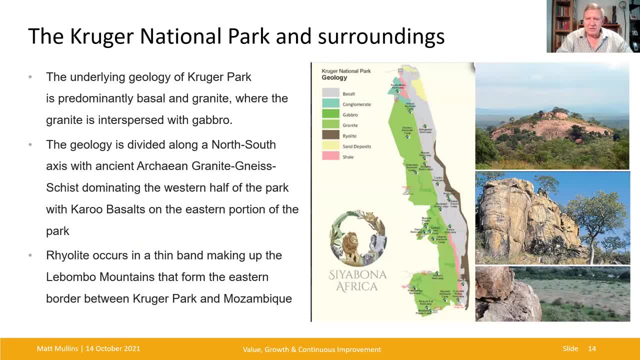 essentially, is comprised of two zones: an eastern and a western zone. when it comes to the geology, and it is on the eastern side it's dominated by basalt and granites, and with western side, it's dominated by archaean granite and gneisses and schist. These form spectacular topography as 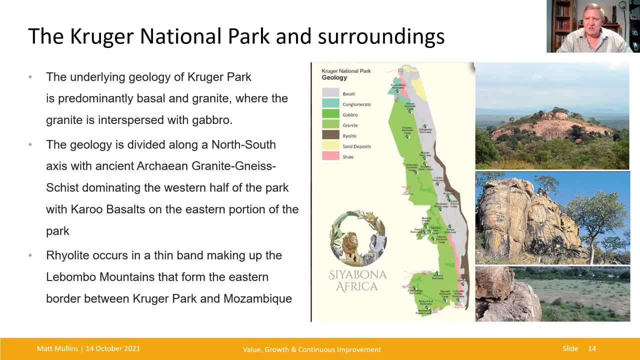 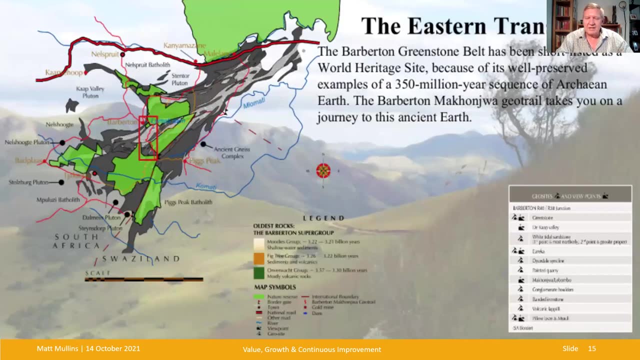 you can see in the in the right hand side and especially down towards the south, you'll see the most incredible topography and incredible geological formations. Moving on to the Barberton area, and this is the place where the Barberton Macondray 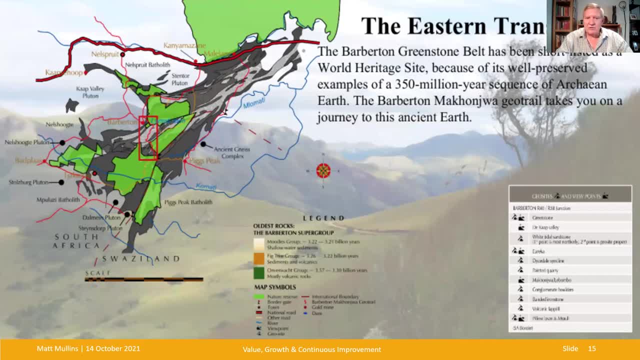 Geotroll Trail has been formed and that is where also gold was first discovered in South Africa, and the scenery is spectacular. It's greener than the western part of the country and there are enormous scenic and historic places to visit if you get a chance to go on that particular trail. 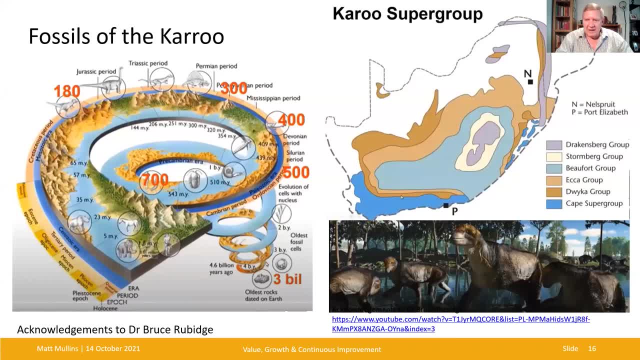 Let's not forget the story of life. Now, I'm not a paleontologist. I would like to refer you to Dr Bruce Rubich and his publications and, incidentally, he is looking at setting up a paleontological center in his original hometown of Graff-Renet. If we look at the development of life on the left-hand, 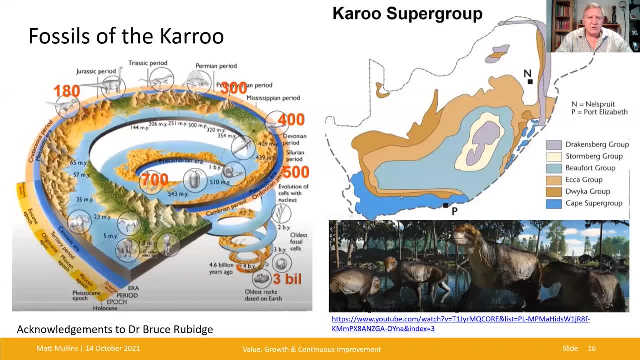 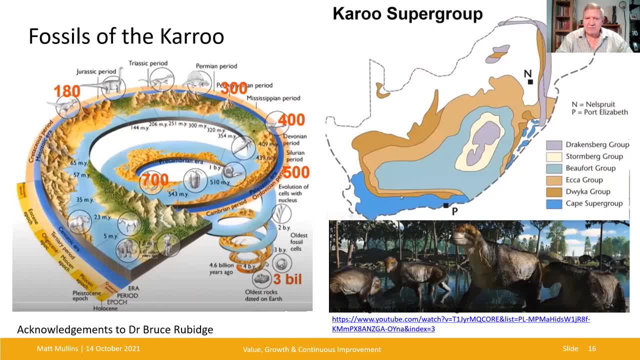 Gondwana land and the number of the fossil record, incredibly rich in South Africa, covering spanning a period which is not easily seen in other parts of the world, all the way from about 500 million years down to about 180 million years, and a magnificent record of 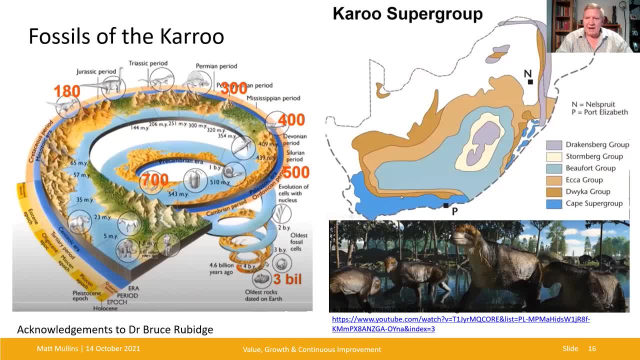 dinosaurs and pre-dinosaur fossils. On the right-hand side it shows quite clearly the enormous dominance of life. Also in the center is a far more ridge of sediment carrying much lighter sediment, but and in the left part of the lower area is a large rằnghaw of sediment carrying a relatively small amount of sediment. 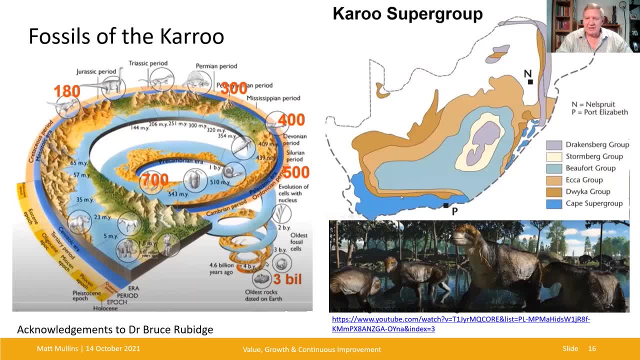 The river makes grow 5-10-��고es or thousands of liters worth of sediment throughout the entire water. The Dubний Highland presents a warm, Blue, überitic falling temperature which is called Pleureen at the bottom 位置, testament mineral's base sediment. just charm by being worth 50 of % of all sediment diameter in the blue Waterfall. 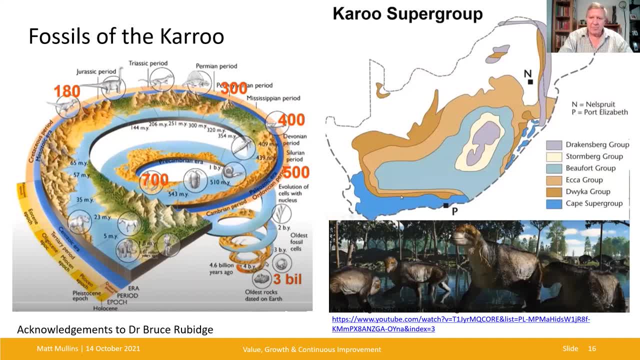 In the blue, perch españolas natural galaxy of the topfour is showing the Cape Super Group, the, Whereas in the blue is shown the cape Super group. he is for Port Elizabeth breakup of Gondwana land itself. This shows you a general scene of the Karoo on the left-hand side. 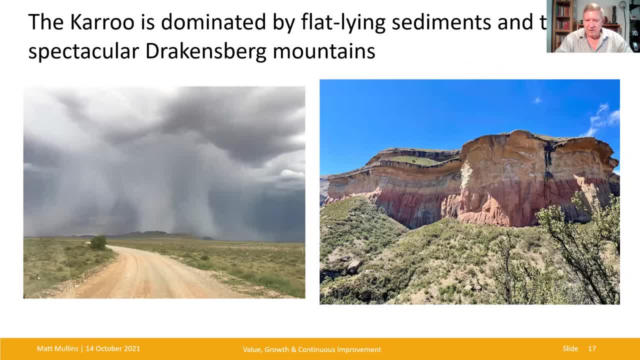 and some of the Karoo Inselbergs, which are the remnants of the dolerite dikes which fed the Karoo sediments. The aridification of the Karoo followed the sedimentation and you can see that in what's called the cave sandstone. 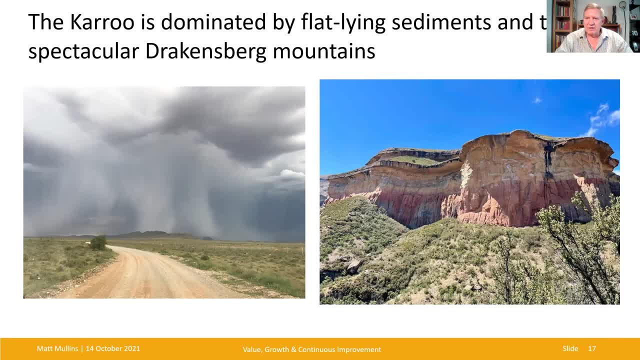 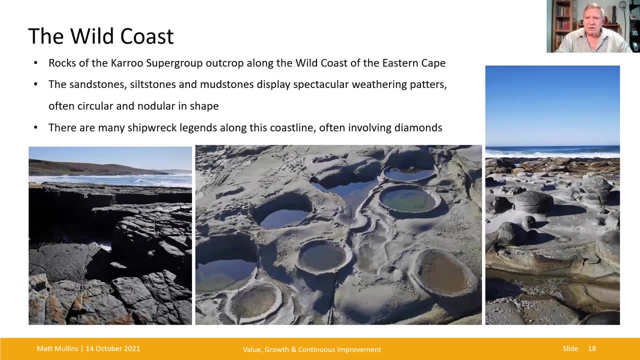 which was formed just prior to the eruption of the Drakensberg Volcanics. If any of you have had the pleasure of walking along the wild coast- and I'll turn to that now- you'll see the most incredible weathering features all the way along the coast in 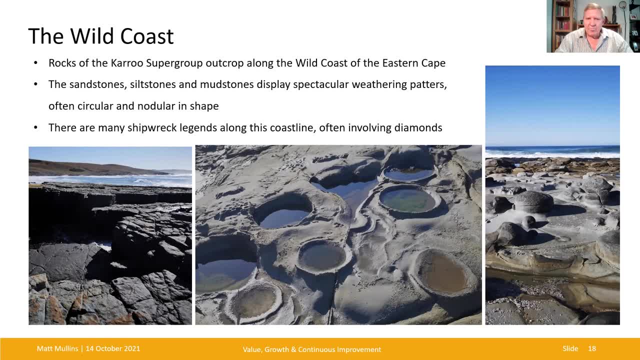 Karoo sediments, mostly of the Beaufort group, and many of them display these very, very, very well developed concentric weathering patterns. they're often circular and nodular, and it makes a walk along the coast an absolute pleasure to see them. As I said before, there are still many. 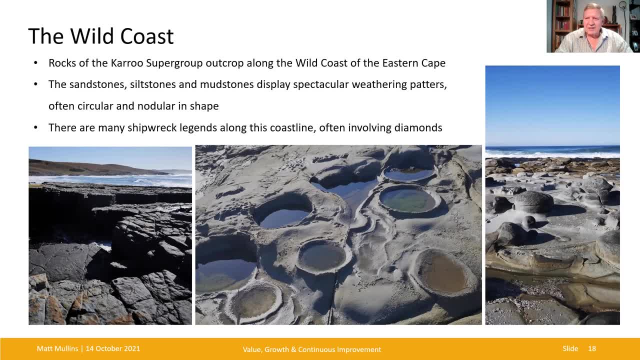 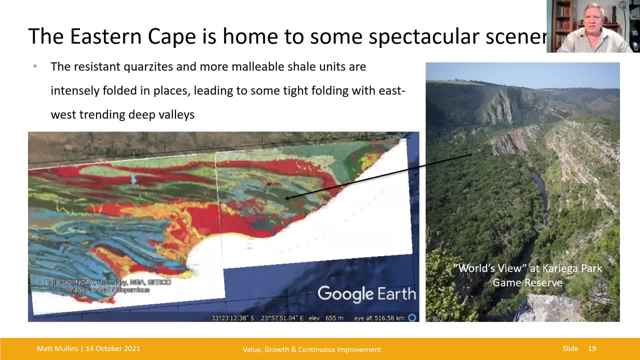 shipwreck legends involving diamonds along this coast, and many of them, I think, have grown with the telling over the years. We turn to the Eastern Cape, and this is where I've been involved in for the last couple of years. it's home to spectacular scenery on the side of the eastern side of the cape: fold mountains. 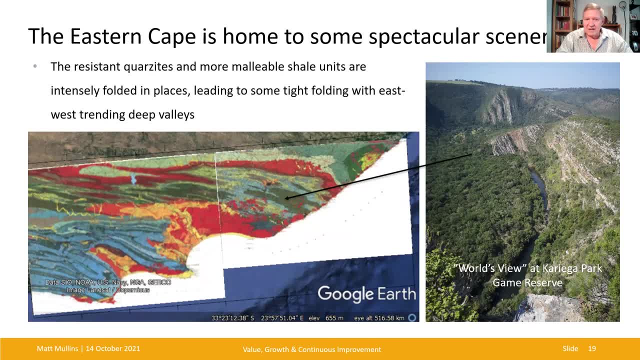 and you can see the east west valleys are largely dictated by the geology. if you look at the left hand side, mostly cape supergroup, but you also have some recent sediments filling in valleys, like in the algoa formation in around port elizabeth. you also would have the enon conglomerate. 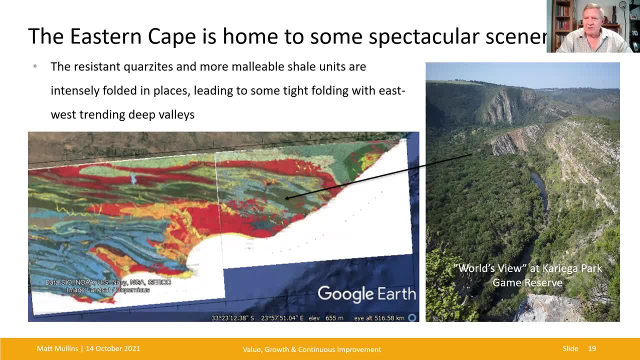 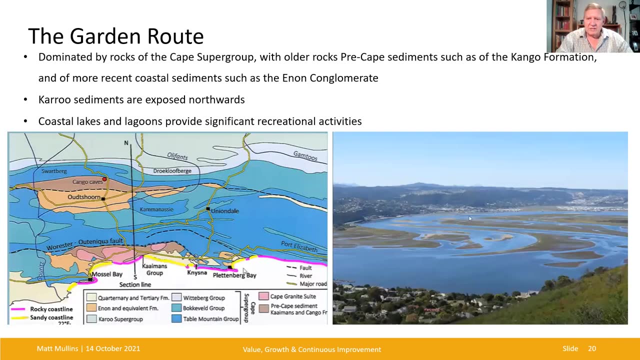 formation close to nasdaq, where it's well exposed on the right hand side is what called world's view, and that's where we've been doing a lot of work with vegasa at the curricular park game reserve. turning to this garden route itself, you have a number of different lagoons and estuaries which 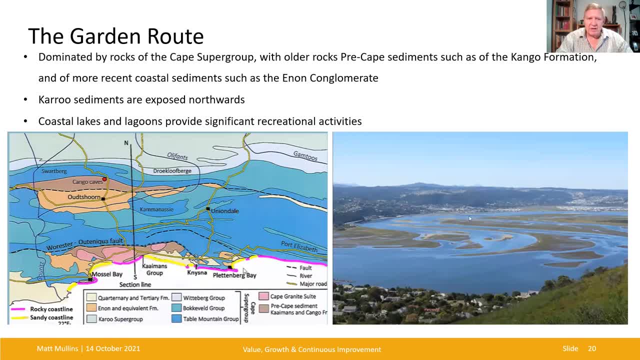 are dictated by the the recent geology of the area. if you take a section from south to north on the left hand side, you'll see you go rapidly from the recent sediments, the caiman's group sediments, into the cape supergroup sediments which are shown in the blue colors. 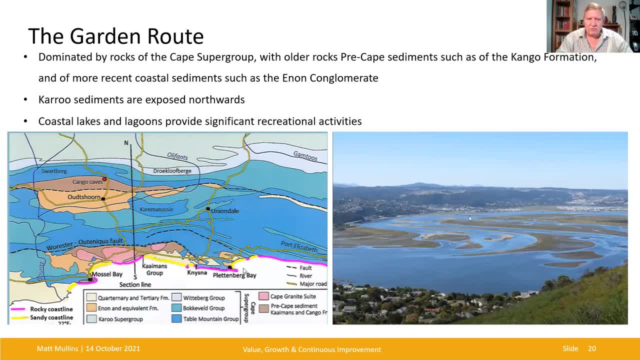 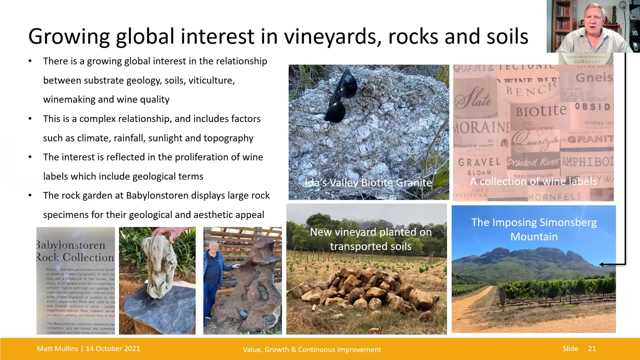 through some- the otsu and karu group- and into the karu supergroup in the north where folding is a lot less and it's a lot flatter and the biomes i have changed considerably. it's move further west and there's a global growing interest in the relationship between vineyards. 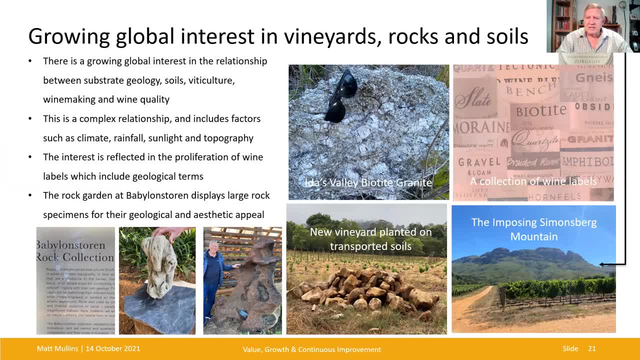 rocks and soils and we can see that in the wine labels that have been developed and you can see on the top right hand side geological terms that have found their way onto wine labels: biotite, moraine, nice slate, obsidian, gravel and fibuliate and others. In the Cape we have a combination of granites, sandstones. 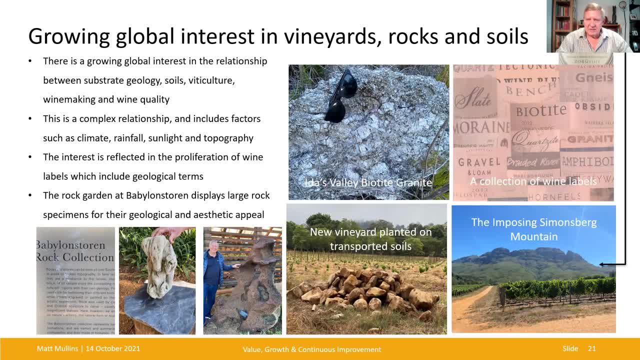 and the Malms regroup schist and the like and a lot of transported sediments in the area In the bottom left in the middle at the bottom is a new vineyard planted on transported soils and the rocks. there are all boulders from the Cape Supergroup. 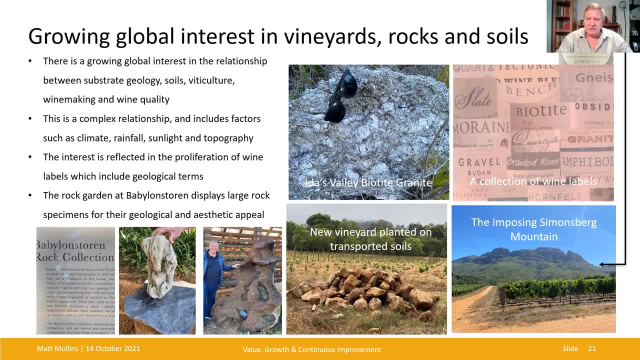 withered off the Simonsberg mountain, which you can see on the right hand side. An interesting aside on the Simonsberg is that there's a defunct silver mine which was operated in the 1640s I think, but it was salted and I think, as far as I can remember, it was the first. 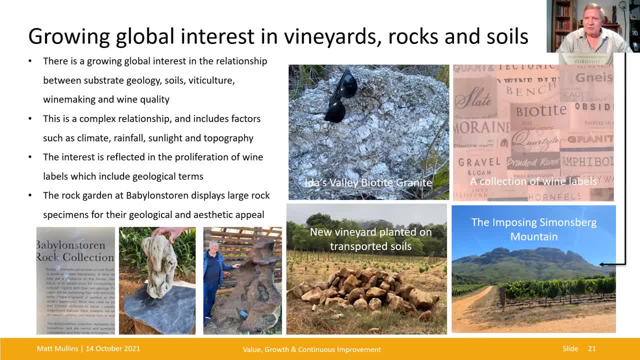 mine to be granted a mining license in the Cape, and also it was the first mine to be salted in South Africa. On the bottom left, for those of you who have the chance to visit it, is the rock garden at Babylon's Turin, where large geological specimens have been chosen, not just for their 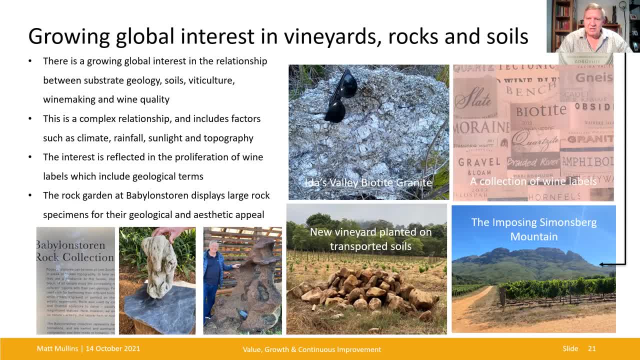 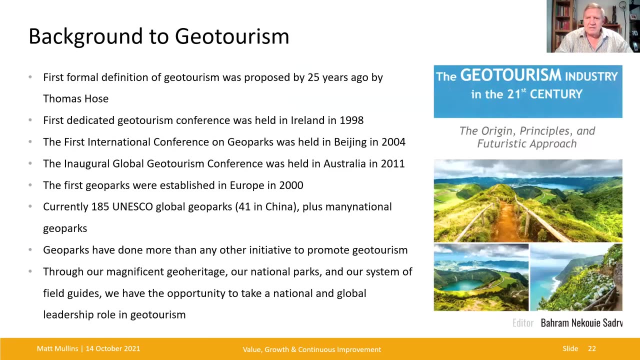 geological interest, but also for their aesthetic beauty, and Nick Norman has been instrumental in helping to develop that incredible rock garden. With that geological journey, I want to go back to geotourism. It is an incredibly fast growing area of tourism. The first formal definition was only: 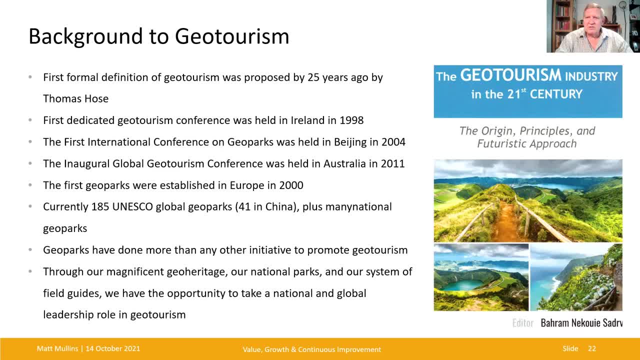 proposed about 25 years ago and the first geotourism conference was only held about 20 years ago and the first international conference on geofarcs was held in Beijing and the first geopark was actually established in Europe in the year 2000. so just 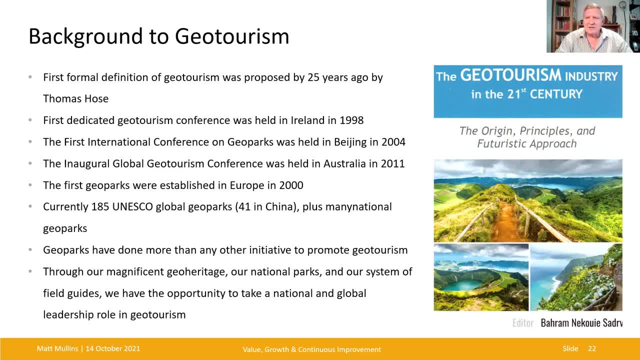 21 years ago. There are currently about 185 UNESCO global geoparks, of which 41 are in China, and there are many national geoparks, and our statement has been made throughout the world and reinforced that geoparks have done more than any other initiative to promote geotourism. 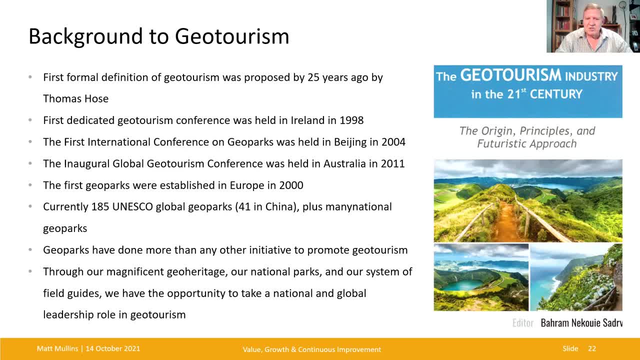 I would like to say that through our incredible, magnificent geoheritage, through our national parks, through our system of field guards, we have the opportunity to take a national and global leadership role in geotourism. We've made some steps towards that. There are many, many excellent. 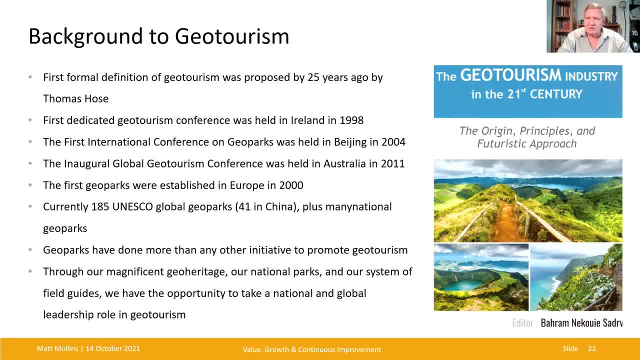 initiatives in South Africa in terms of the development of geoparks, geotrails, geosites and the, and many, many different publications that we can see describing the various geological superlatives in South Africa. We, in particular, are involved with FGASA in developing. 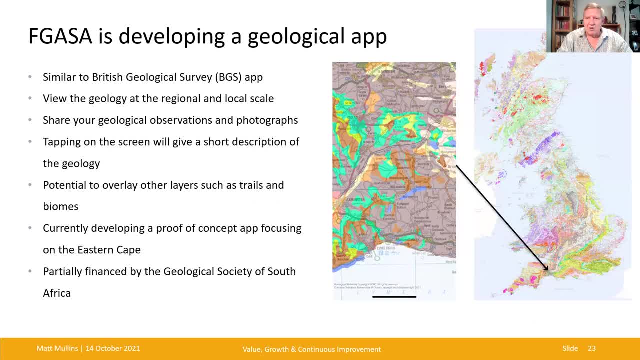 field guards for our South African game parks or our South African national parks, and mainly in identifying the areas of interest and in developing those field guards towards developing a specialist field qualification in geology. Part of this has been our initiative to develop an app whereby we can 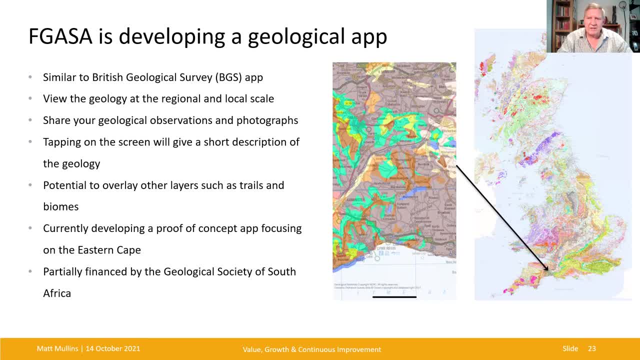 actually not only look at the geology of the particular area that we're in, which would be available to everyone who would be in those parks, but also which would be available for individuals to use. So we've been working with the field guards and tourists themselves to actually 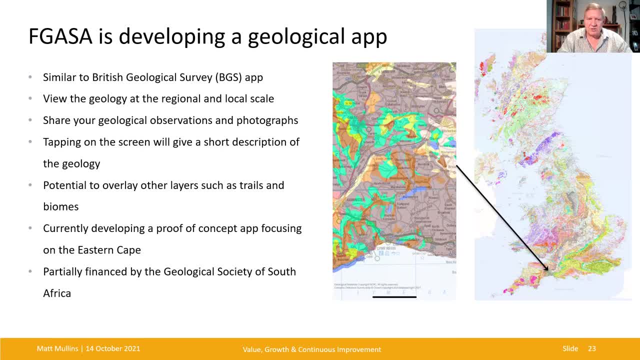 supplement the particular app through the inclusion of photographs and observations on it. We're currently completing the proof of concept and of this particular app and of the field guard approach, with a view towards getting a prototype out by April next year, and I'd like to just 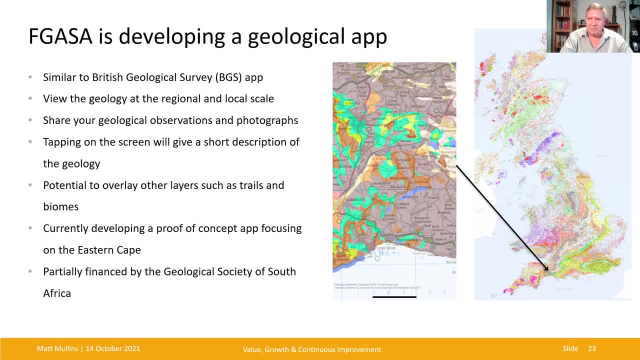 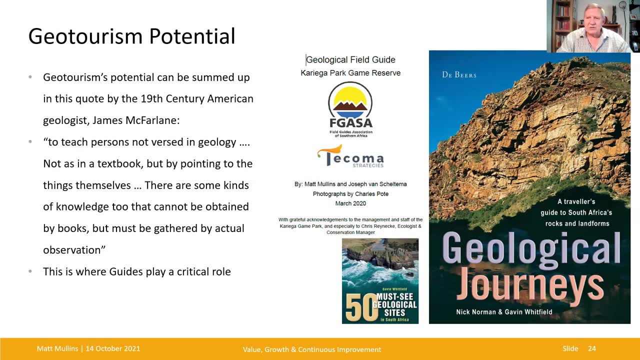 acknowledge that this has been partially financed by the Geological Society of South Africa and the National Geological Society of South Africa. Thank you, Thanks to them. To finish off there, geotourism has an incredible potential. It has the potential to add jobs, it has the potential to attract tourism and it has the potential to involve. 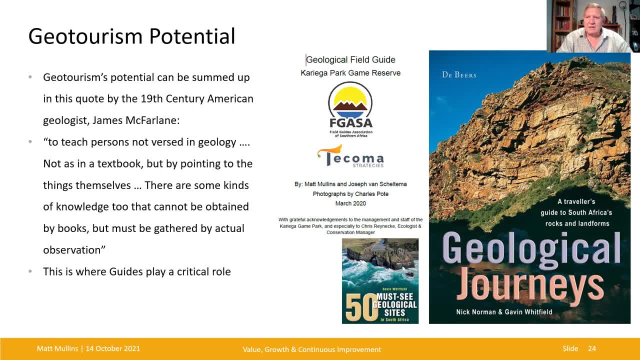 local communities as well. However, it's not something that you can learn in a textbook, and this is where field guards are so important. There's something that you have to demonstrate out in the field. What is that? How does that particular land form? how does it form? 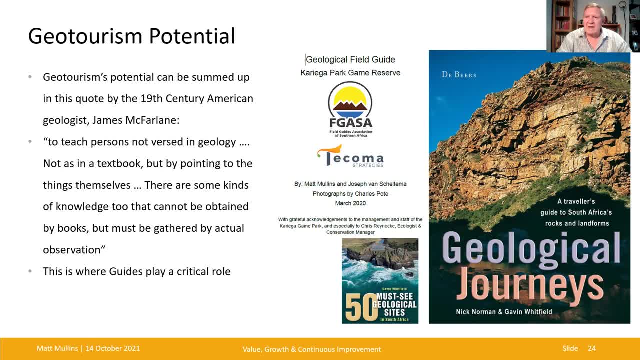 What does it do? What rock is it made of? How does it fit in with the vegetation, How does it fit in with the animal life? All of those sort of questions are ones that we need to talk about, and talk about with ourselves and in the field, amongst the tour guards and amongst 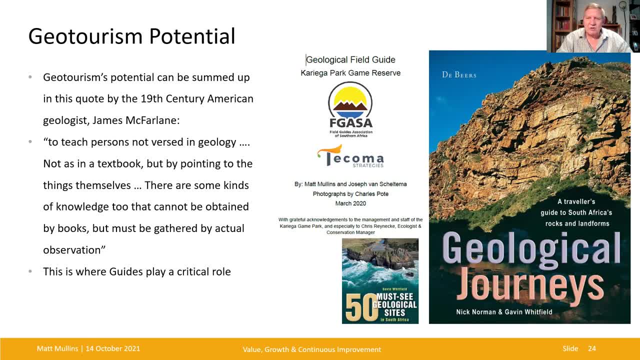 the tourists themselves, And so I'm looking forward to a very, very good future working with Fagasa in helping to develop this and hopefully helping to get more and more people involved in the development of geotourism in South Africa, and I'd like to say that you, as guides, play a critical 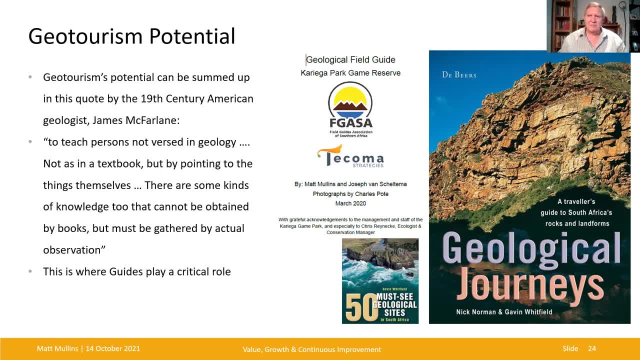 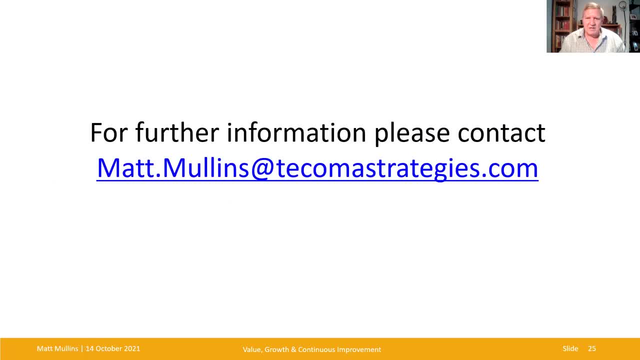 role in helping develop this particular area of tourism. With that I'd like to say thank you, please. and there is my address, my email address. please get hold of me if you'd like to talk to me further or if you'd like to have any further questions. 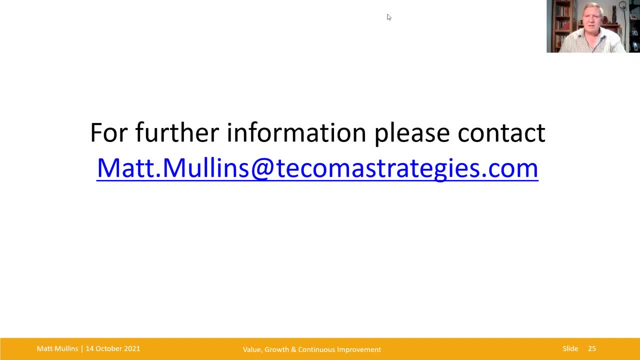 with that, i'd like to stop my share and finish off the recording.